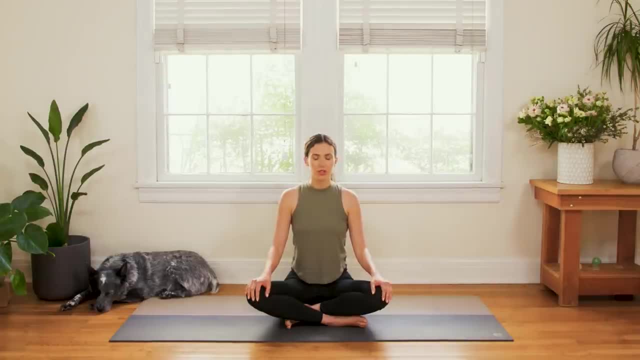 relax the shoulders and just take a second here, if you feel comfortable to close your eyes and sit up as tall as you can and know that this time is already valuableso you don't have to nail the seated posture. it's not always important, but I hope so. 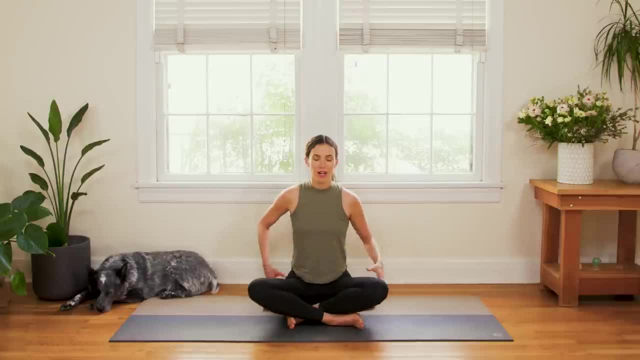 posture. if your knees are hiked up, if your tips are high- or your tips your hips are high, your low back is tight. just know you are not alone, But we have to start somewhere and a good 10 minute practice is. 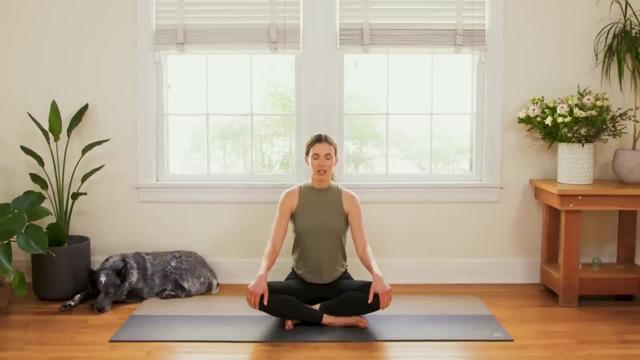 an excellent place to begin. So close your eyes, Accept where you are today and thank you so much for being here. Take a deep breath in through your nose- Nice and easy- And a long exhale out through your nose or mouth. You can totally choose. 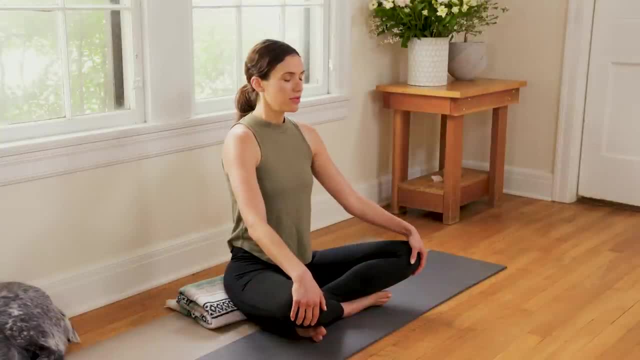 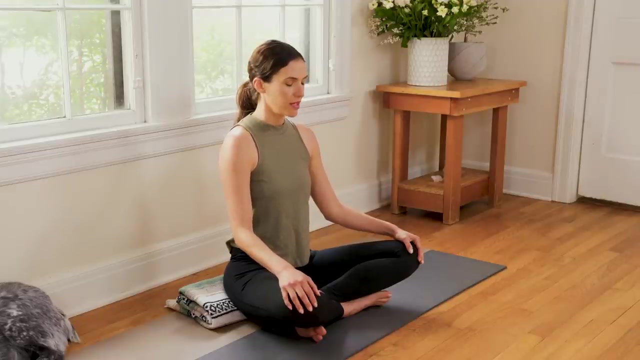 Just move intuitively here with your breath, Inhaling in deeply And exhaling out through the nose or the mouth, Your choice. And again, deep breath in And long breath out, And one more time, Deepest breath You've taken all day. 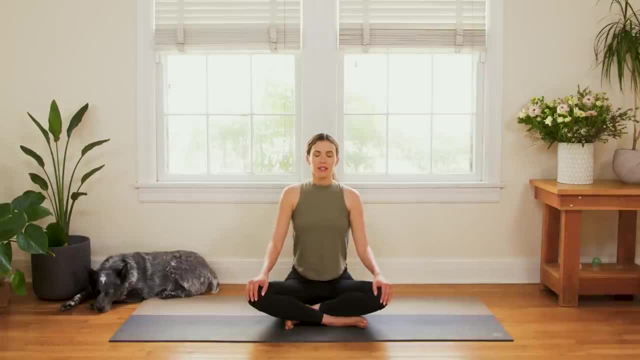 Deep breath In And out Nice. Now continue to breathe deeply. You don't have to match those big inhales and big exhales, But whatever it means to you, you want to just keep an awareness of your breath, So don't let it drop. 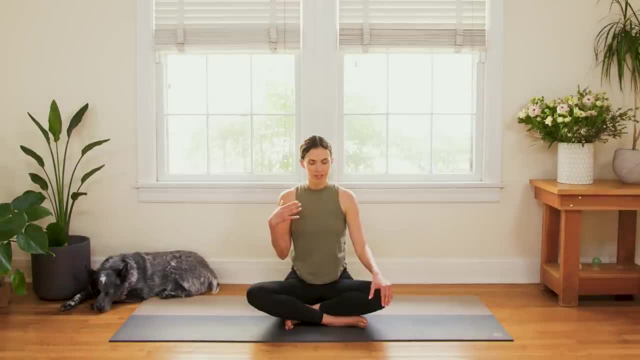 Drop back into that unconscious breathing pattern that we often move throughout our day. in Best, you can allow your yoga practice to be about conscious breath, this constant, even if it's small awareness of how you're breathing. If you keep that up, you're gonna have a beautiful 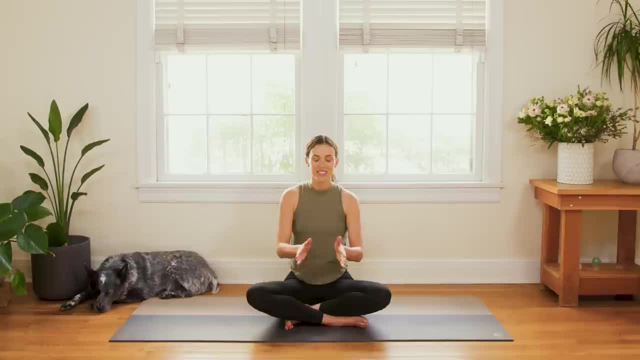 practice. Alright. so hands come together. next, Palms at the chest, Or the heart space. We call this Anjali Mudra And we'll just drop the chin to the chest here And there is a moment to kind of connect to your heart space, or 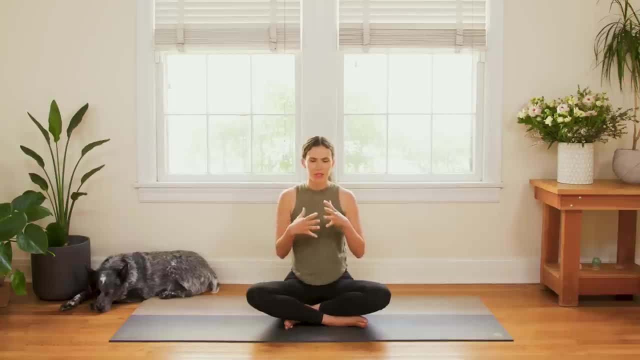 your emotional well-being, And if that's not really why you're here or that doesn't feel comfortable for you, just enjoy this awesome stretch in the back of the neck. Yes, And if you're like me, I'm like I'll take both. 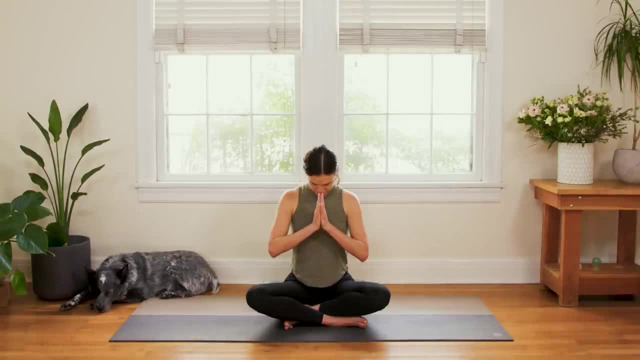 You can just take a quiet moment here And then slowly lift your chest up towards your thumbs And just see if that allows you to sit up a little taller longer through the spine. If not, that's okay, We'll take one more quiet moment here. 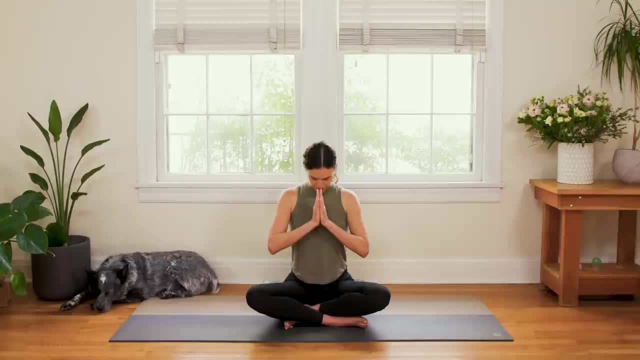 Just finding stillness And expanding our awareness of our breath, how we're breathing, And you can take in any sounds that you hear around you And start to notice how you're feeling. today, This time on the mat, yoga is actually not about accomplishing. 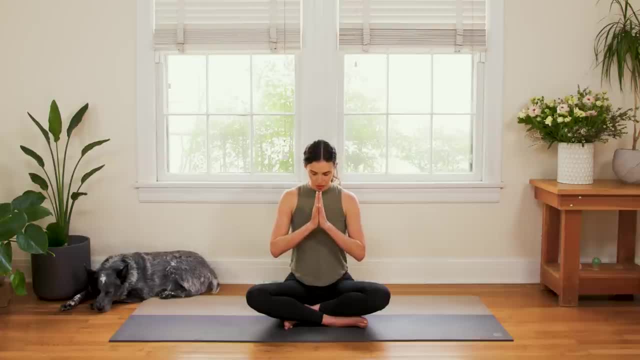 kind of what you think yoga is supposed to look like or feel like. It really is all about you being honest with your experience and taking in your surroundings, Becoming more present with what is. Let's take a deep breath in to transition here together. 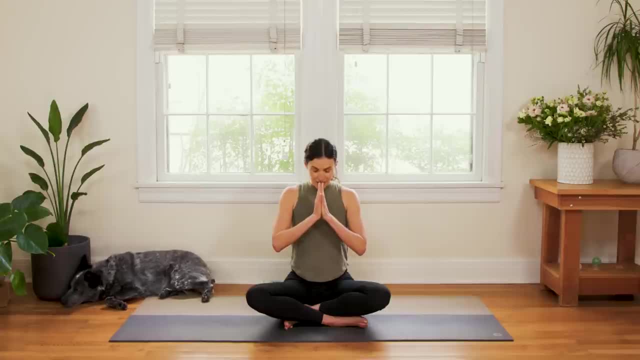 Inhale And exhale to open your eyes, release the hands And we're just gonna bring the fingertips to your sides. So we're about to come to all fours. So sit up, nice and tall, Draw your navel in and up. 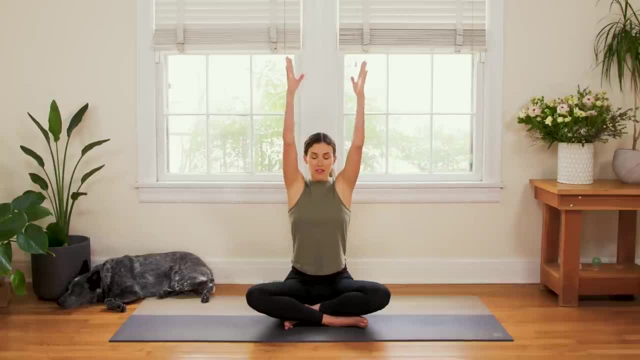 And inhale. reach the arms all the way up and overhead. Fingertips kiss together or they can just reach up towards the sky. Get long, long breaths, Get long through your side waist And think about drawing energy up from the base of the pelvis. 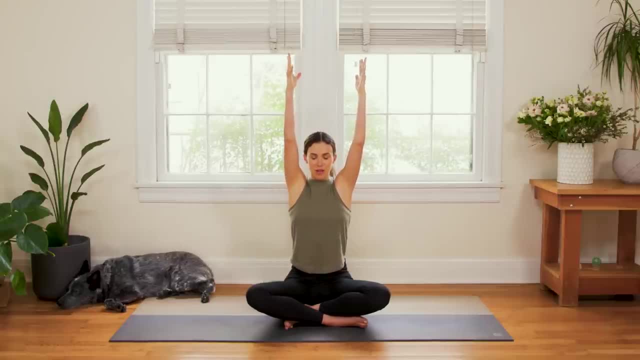 Whatever that means to you And see if that kind of changes the way you embody the shape. Good, then inhale. If it's alright with the neck, look up And then exhale. flow the fingertips down. We'll do that twice more, but a little faster. 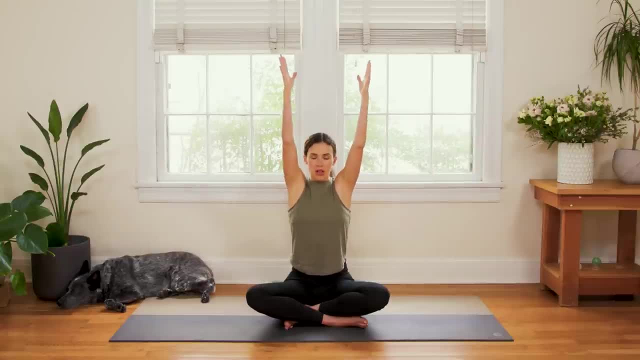 Inhale, reach up, Big breath, big stretch, Long side body Engage, Lift from the pelvic floor. Just play And then exhale, float it down Last time: inhale, reach, lift, See if you can lift the muscles of the pelvic floor a little. 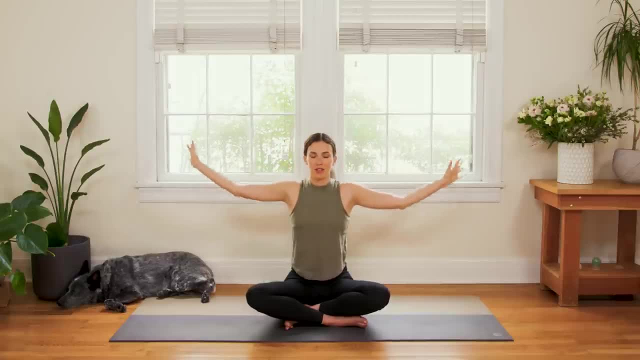 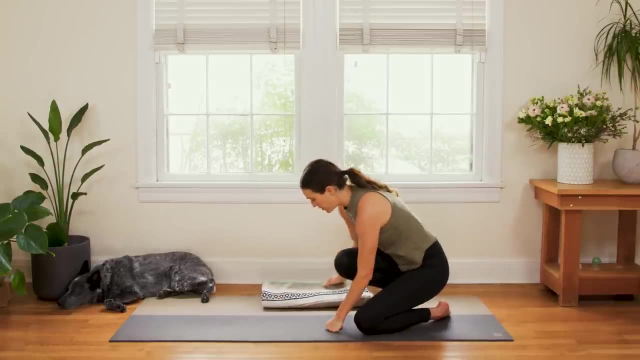 Reach, reach, reach. Find that support from within And then exhale, float it down. Awesome, come forward, We're gonna come to all fours. We're gonna use that blanket or towel- if you brought one- for a little padding on the knees. 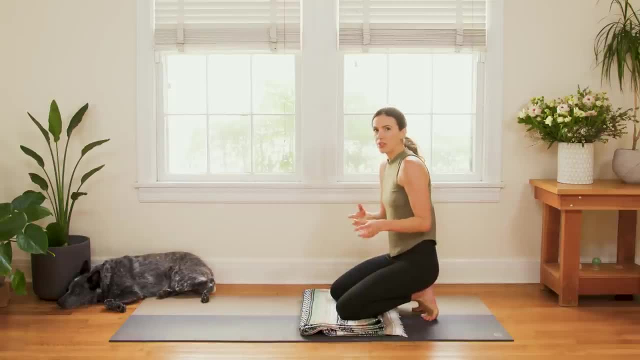 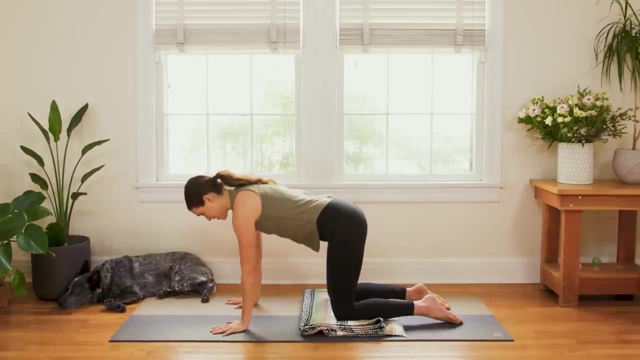 Take your time transitioning. If I'm ever moving a little faster than your body wants to move, obviously listen to your body and really celebrate that relationship that you're honing in on here with the yoga practice. Knees come underneath the hip points. 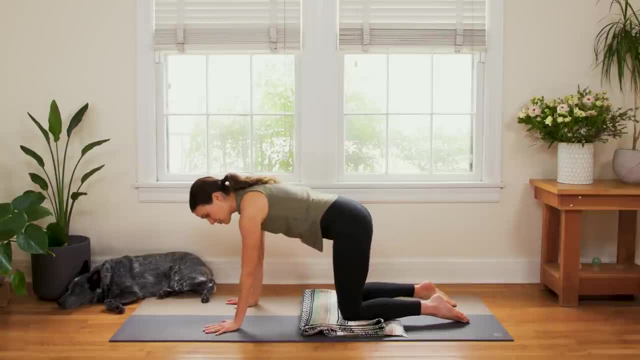 So we're stacking the bones always from the ground up And wrists come underneath the shoulders- same thing. Spread your fingertips wide, Really feel that stretch, And then just allow your front body, the weight of your body, to collapse down here into the 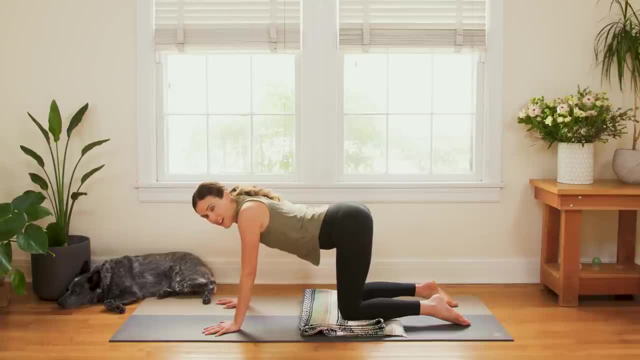 earth, just like me here. So just let it all hang. Now we're gonna start with the feet Press into the tops of the feet Press. just imagine pressing into the shins and then start to lift your belly up and lengthen your lower back. 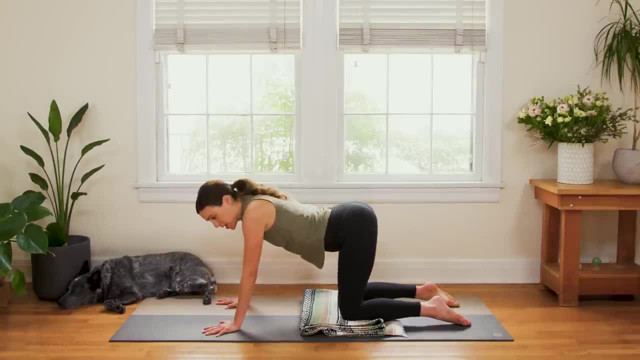 If you're curious as to what I'm talking about exactly, you can peek at me. I'm gonna go from here in this state of just kind of collapse to engaging, bringing awareness. to lengthen my low back: Now draw your navel up. 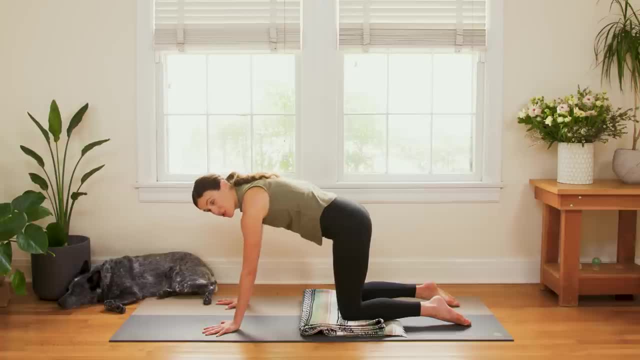 Send your chest up towards the ceiling, Feel your shoulder blades kind of move left to right, broadening through the upper back, And then the last bit is to press into the hands and remember that your neck is an extension of the spine, So your neck might be hanging here like this. 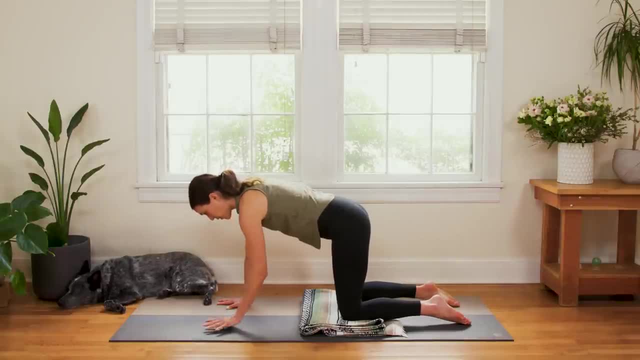 You wanna lift and lengthen through the crown of your head forward, so that now you have this beautiful line from the crown of the head to the tibia, The tip of the tailbone, Great Tabletop Position. Drop the belly now all the way. 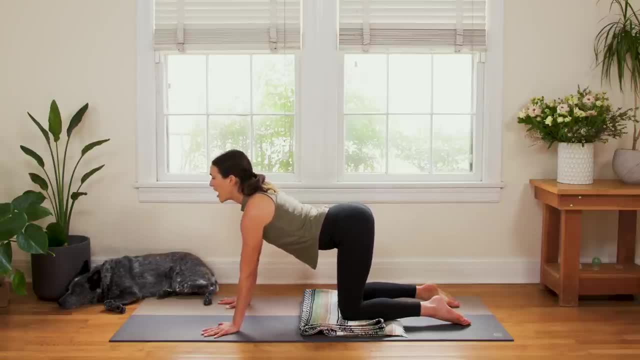 Open the chest, look forward Cow Pose. Exhale round through the spine. chin to chest Cat Again, drop the belly. Open the heart forward. Exhale round through the spine. Twice more Nice and slow. 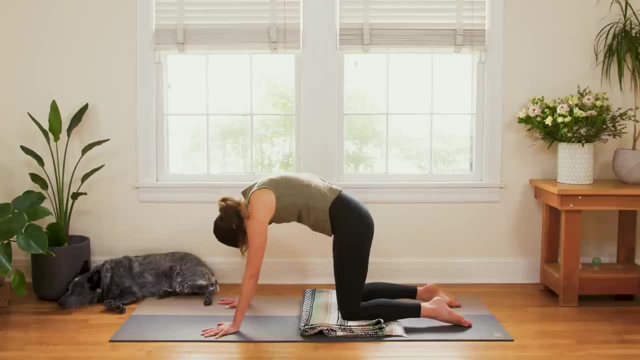 Moving the spine, But starting to really work on this strong foundation, this base that you're gonna continue to build and grow your practice from Great. come back to that Tabletop Position. So nice, neutral spine. Then, nice and slow, we're gonna send the right heel out. 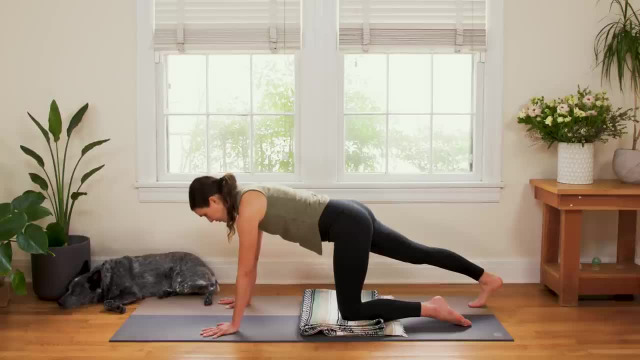 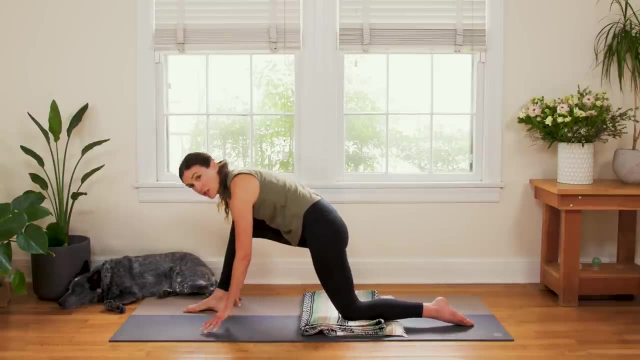 straighten the right leg to just stretch through that right leg, right foot. Then you're gonna step the right foot all the way forward And it may take a couple steps to get it all the way up so that you're in a nice low lunge. 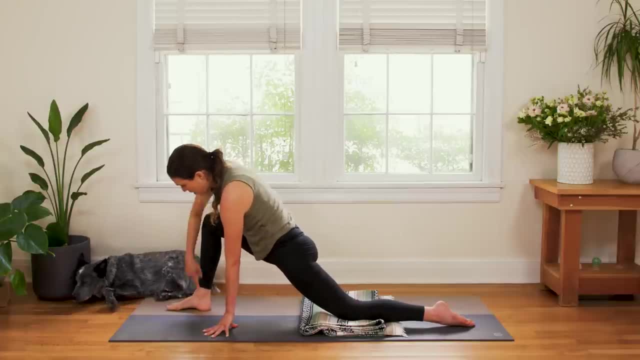 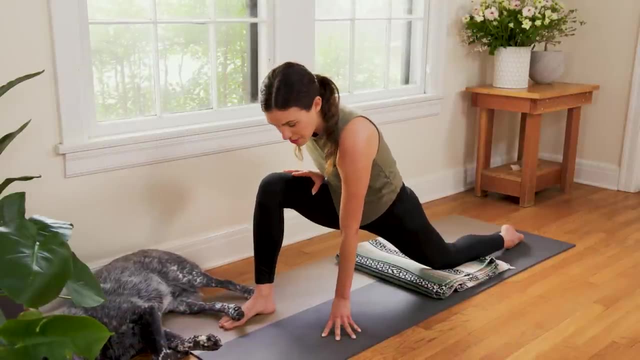 From here we're gonna make sure the right knee is over the right ankle, Again, always looking to stack the bones from the ground up. Then right hand comes to the top of the right thigh, We're gonna press into the back foot firmly as our foundation. 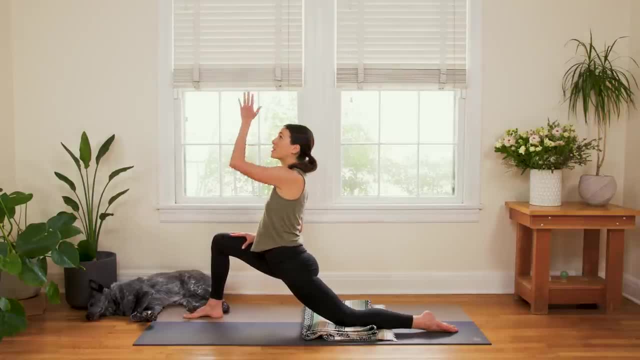 Find that lift from the pelvic floor that we did in Cross-Legged and reach your left fingertips up towards the sky for a little modified low lunge. Inhale in deeply here. Inhale in deeply here. Lift the chest. find length through the crown of the head. 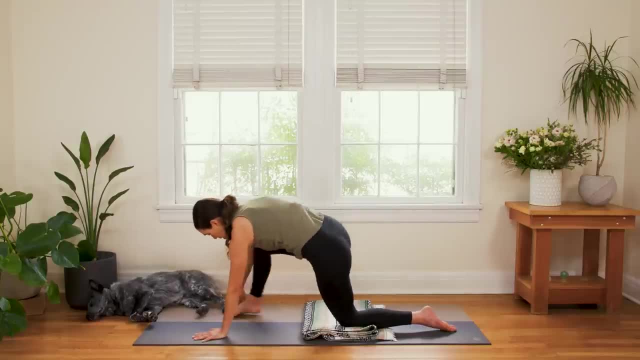 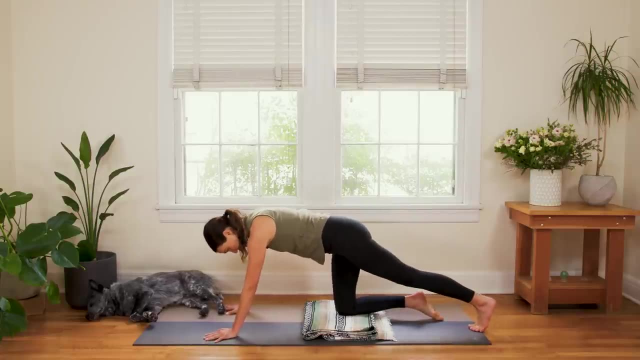 And then exhale, release Hands, come to the ground, We bring the right knee all the way back to the mat or the blanket and we're gonna just do the same thing on the other side. So send the left heel back, stretch, stretch, stretch. 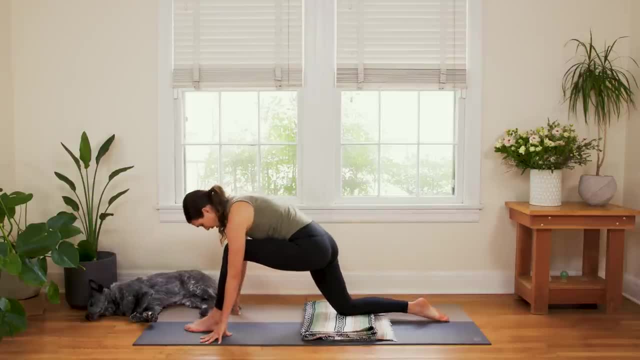 Work that left foot all the way up, Come into a nice low lunge Front knee over front, ankle toes pointing forward. Here we go: Left hand to the top of the left, thigh Inhale, reach the right fingertips forward, up and back. 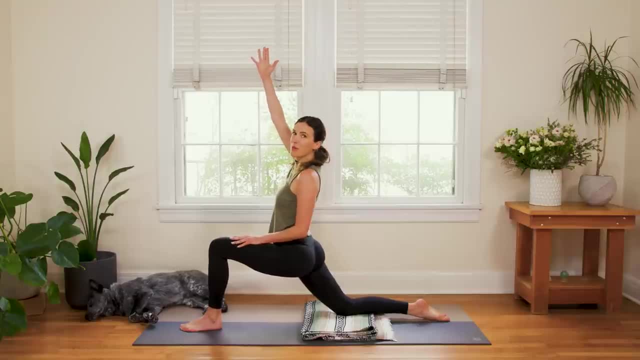 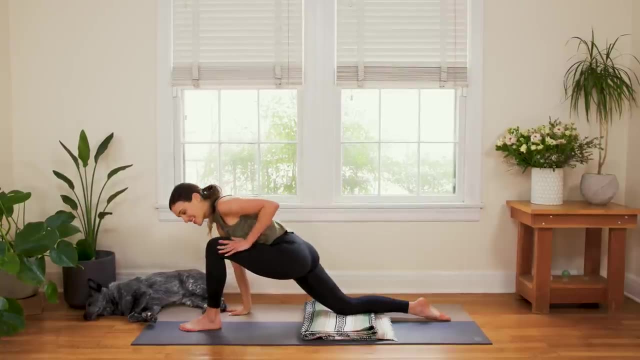 We're pressing into that right foot for stability. We're lifting up from the pelvic floor. Inhale big stretch And exhale to release Hands. come to the mat, We'll bring the knees back down. We're gonna end in an Extended Child's Pose here today.